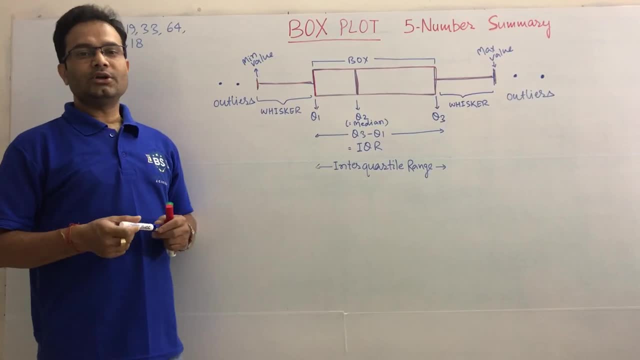 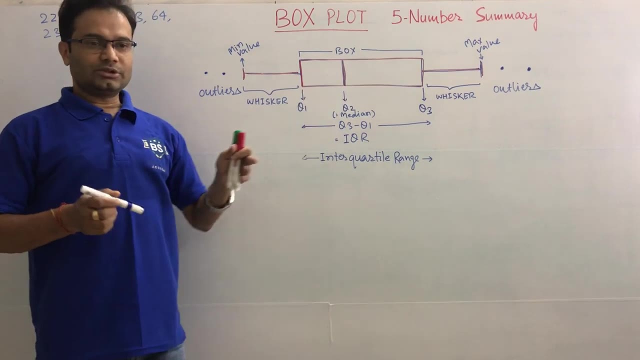 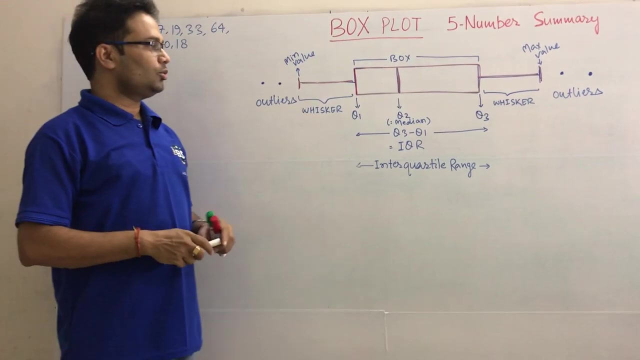 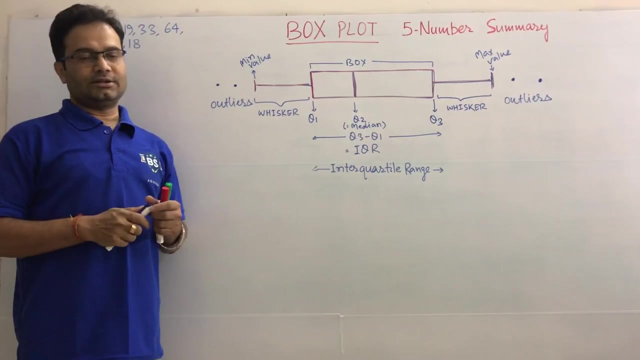 Actually, box plot is a standard way to display the distribution of your data on the five number summary. So suppose if you have some data set like this kind of data set and you want to know what is the distribution of this data means how the data has been spread out in the data set. 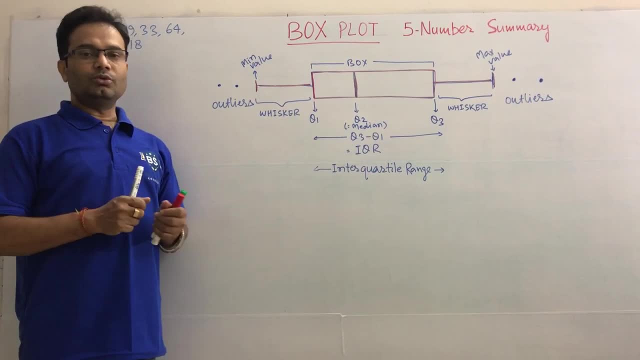 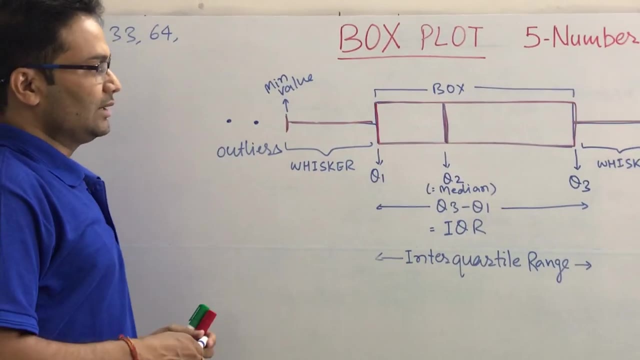 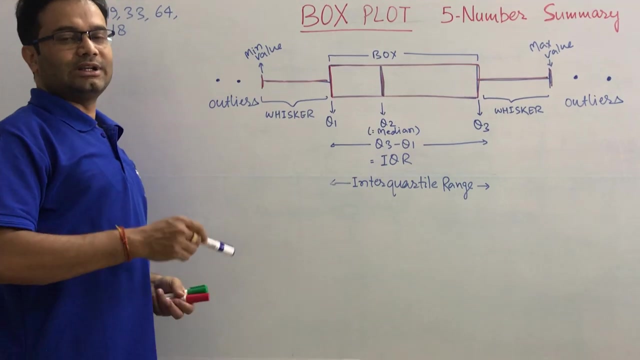 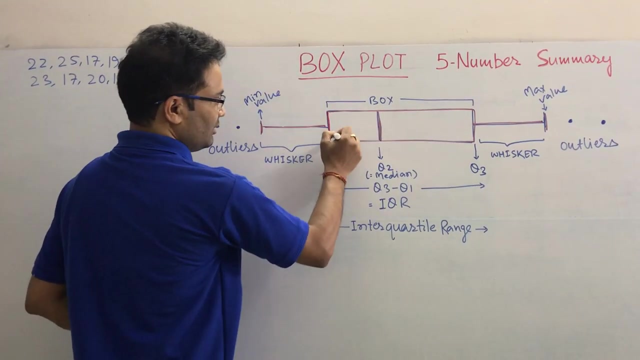 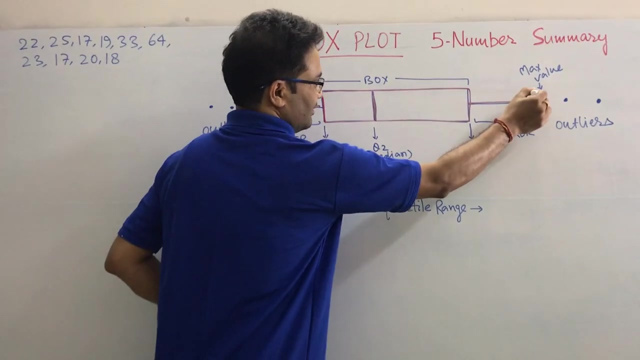 Then box plot is a very good tool to understand all that. So how to do that? Before that you should understand what are the different parameters or different points are there in the box plot. So actually in this picture, if you see, this is the box plot. So one rectangle box, two lines both sides and this two lines ending line. So this is the box plot. 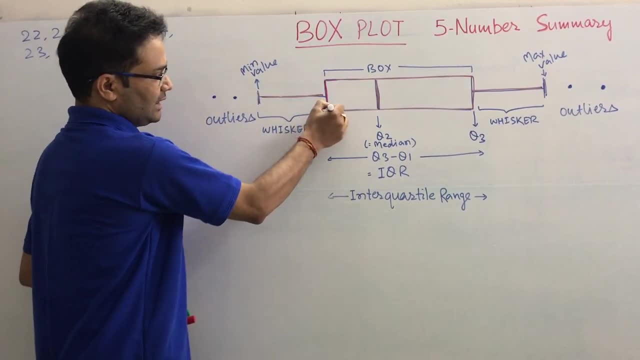 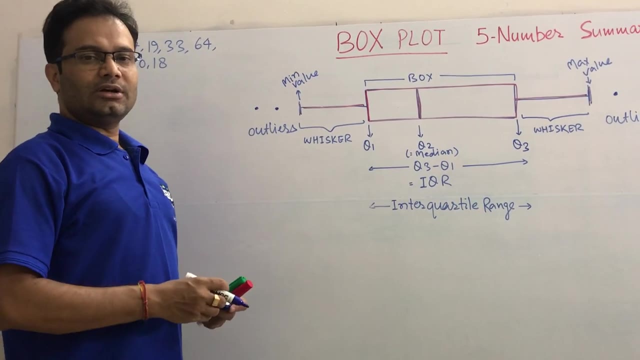 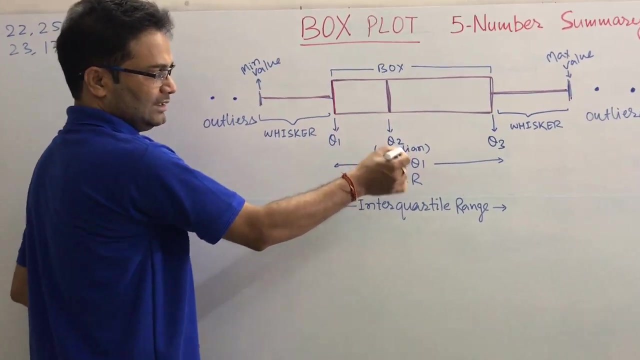 So this is the box plot. So this one, the starting of the box, is the Q1.. Q1 is the quartile, first quartile, and you can also say the 25th percentile. This middle line is the Q2 percentile. Q2, that is the median, that is the middle part of your data set, and this is the third quartile. 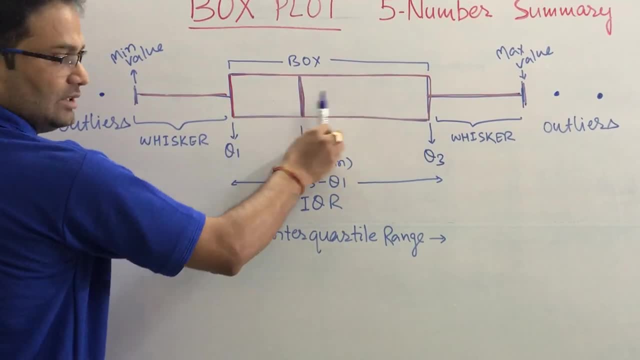 So 1,, 2,, 3.. Apart from these three, you will get the mean value also. So 1,, 2,, 3.. Apart from these three, you will get the mean value also And you can get the max value. 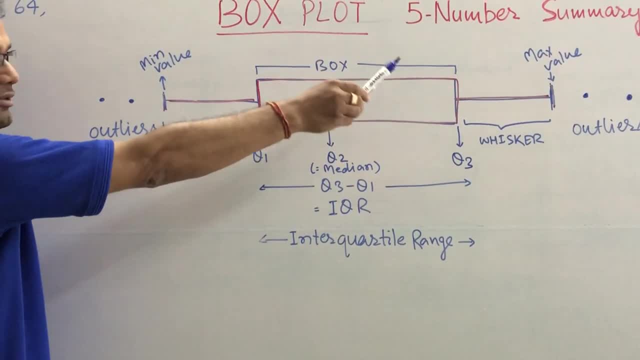 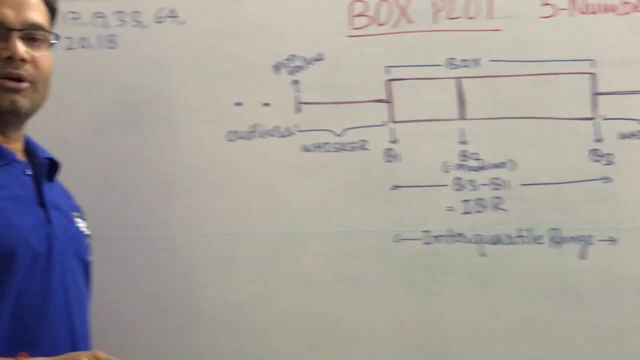 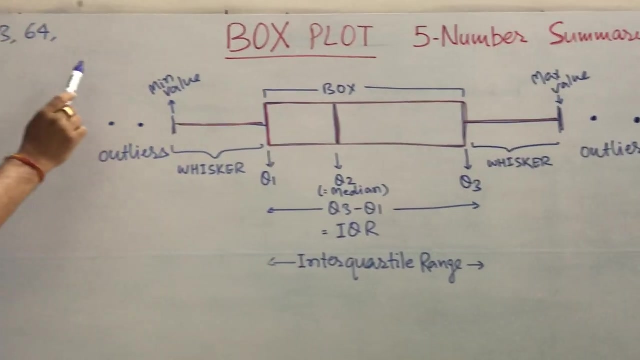 So that's why this is called the five number summary: 1,, 2,, 3,, 4 and 5.. Apart from these, we can also get the outliers. So if any outliers are there in your data set, you can find out in the box plot and what is the outlier. 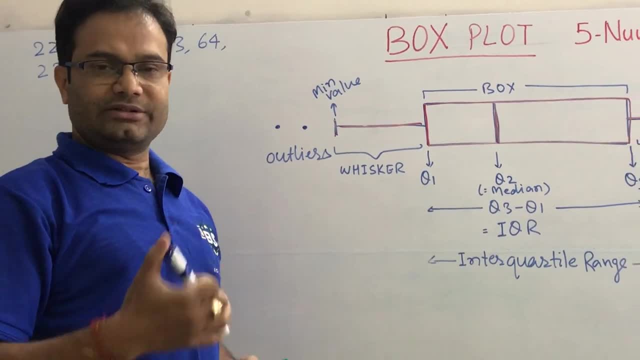 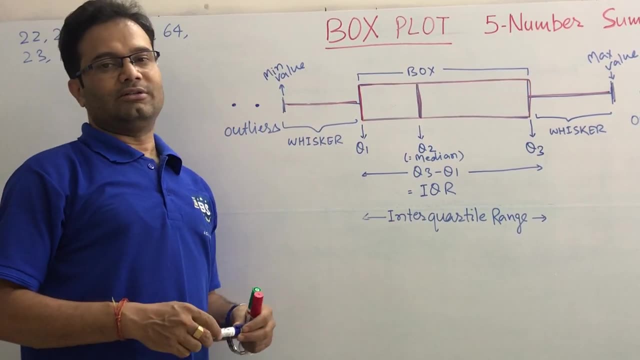 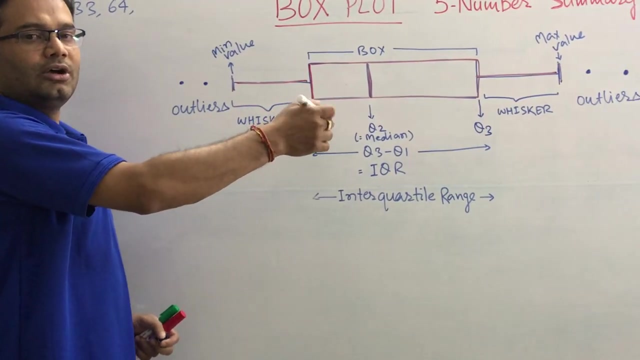 Any data That is by characteristics. It is different from the above, from the other data in your data set used to call the outlier. so after viewing the data you can't say which is the outlier. but i will show through the some formula how you can find out the outlier. 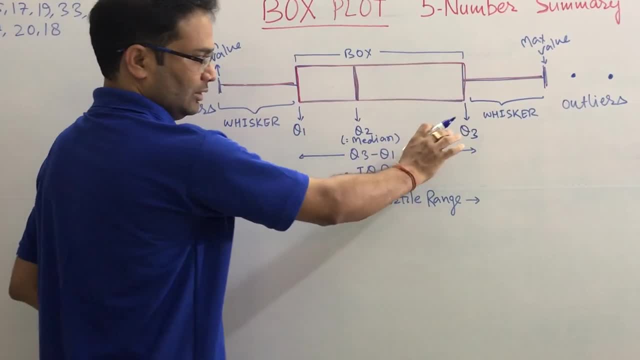 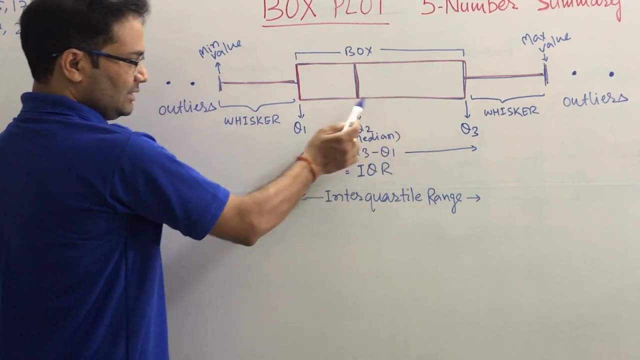 so now you understand the q1, q2, q3 will you show. i will show how to get it. what you think is if this is the q3 and if this is the q1. so if you differentiate, you can get the q3 minus q1, so the 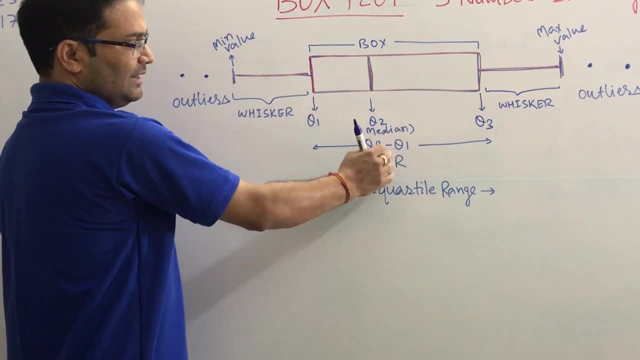 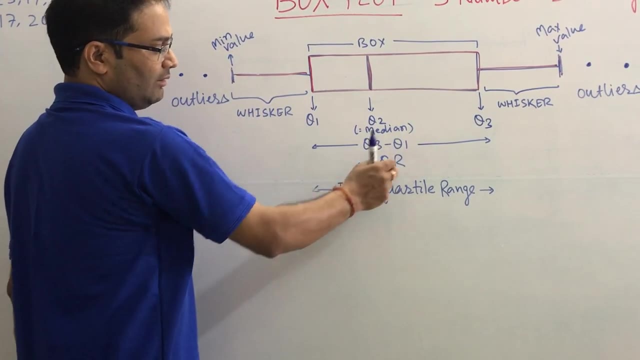 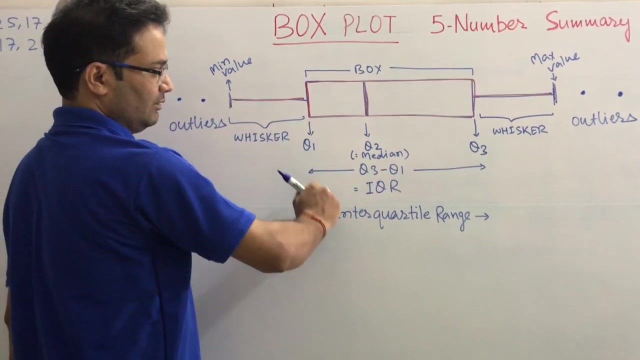 value of this box would be the difference of the q3 and the q1. okay, and that is called the iqr interquartile range. this is important factor. it is very much useful to find out the outlier. so interquartile range is equal to. 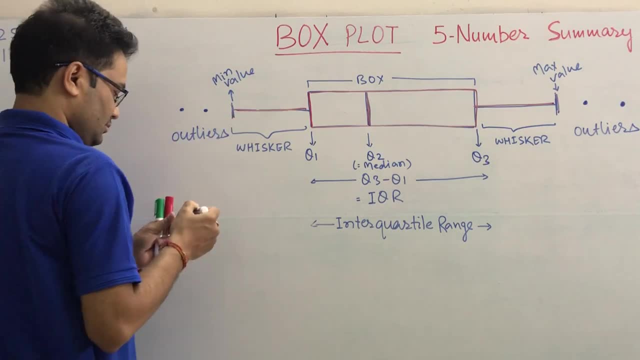 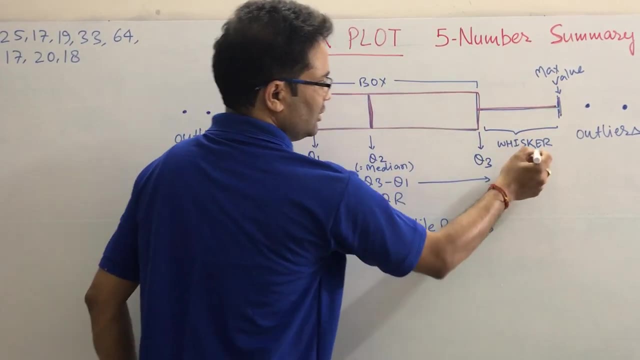 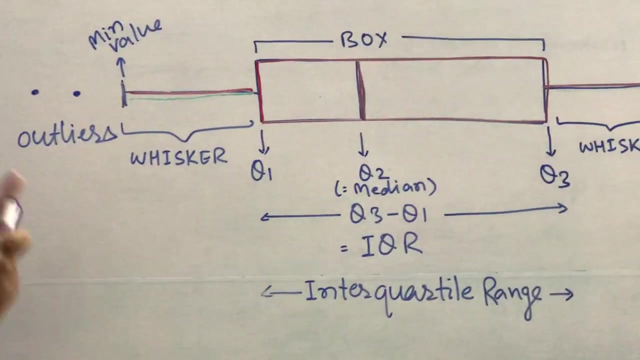 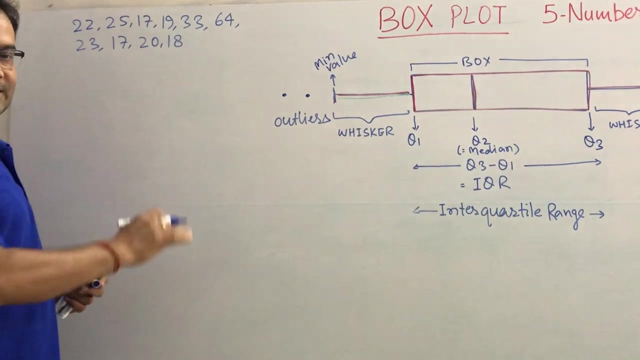 q1, q3 minus q1 and these two lines, if you say in the green color, these two lines are called the whiskers, these two lines. okay, so let us start how to construct the box block. so suppose you have given the data. so first what you have to do. you have to arrange the data in the ascending 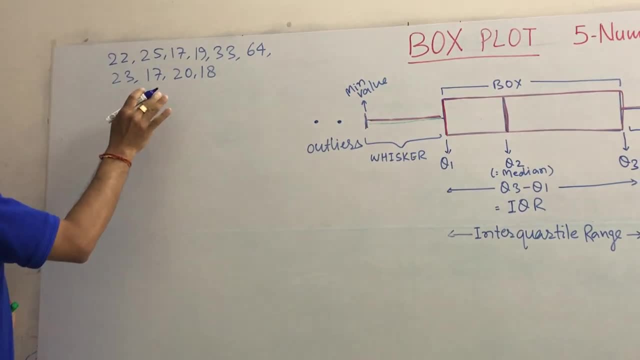 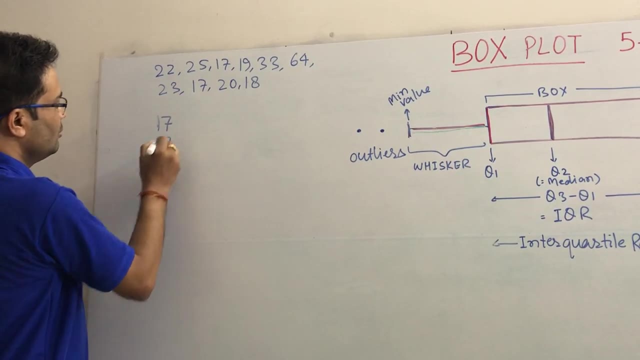 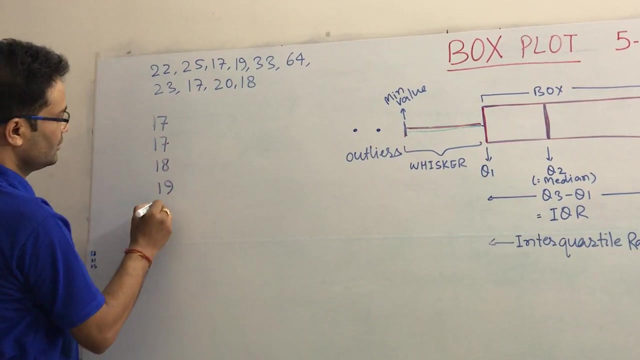 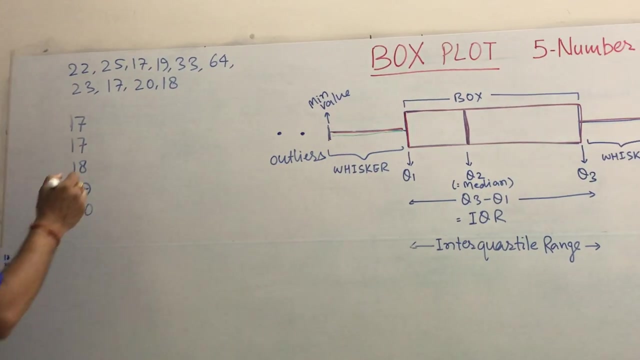 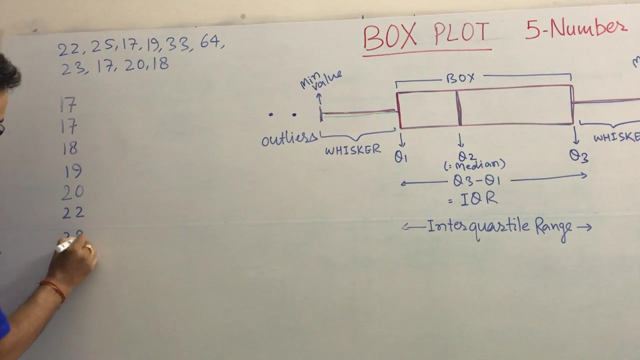 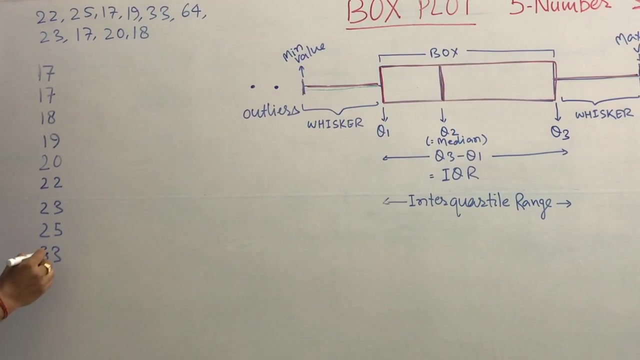 formula. so take the latest, the lowest data here: 17, one more 17, 2, 17 is there, then 18, 19, 20, then 22, 23, 25, 23, 25, then 33, then 64, then 64. so easy way: when you take the data, just cross it 17. It is easy when its cross it 17, 17 i took. 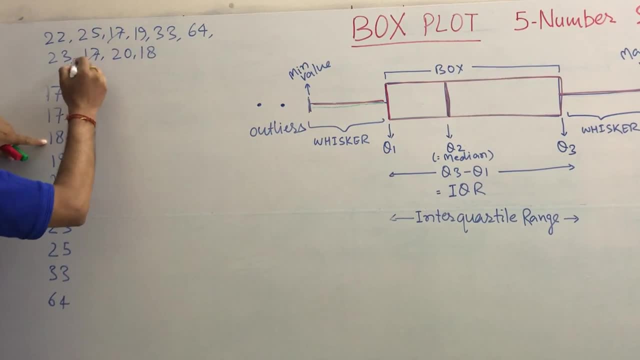 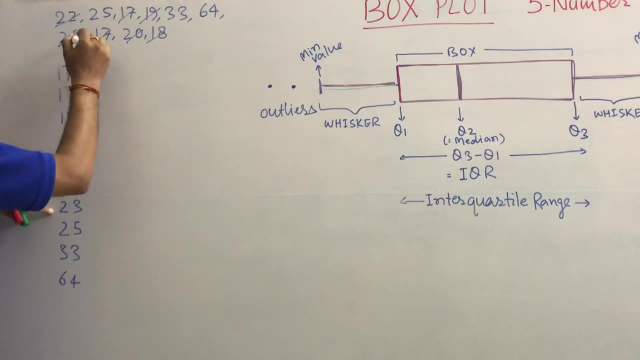 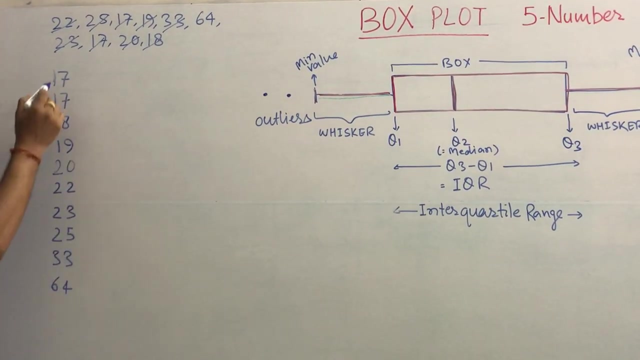 17, 17, 17. i took 19,, 22,, 22, 23,, 25, 33 and 64, 10 data again cross 3, 2, 4. i will not cross here now because let me see on me, because let me have a look at this box here. 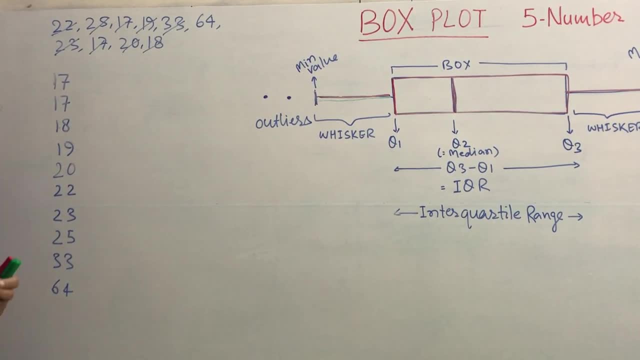 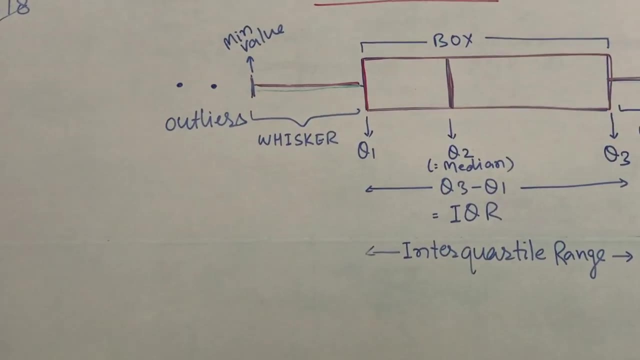 5, 6, 7, 8, 9, 10. so i got the 10 data. so how to get the median median is the thing. this is the second part. i how to get the median. so now, what is the median number? so here, number are the even. 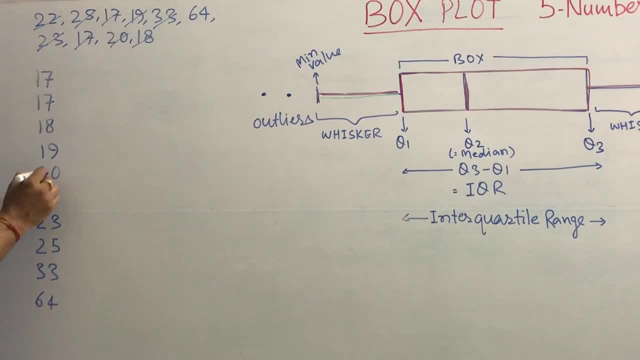 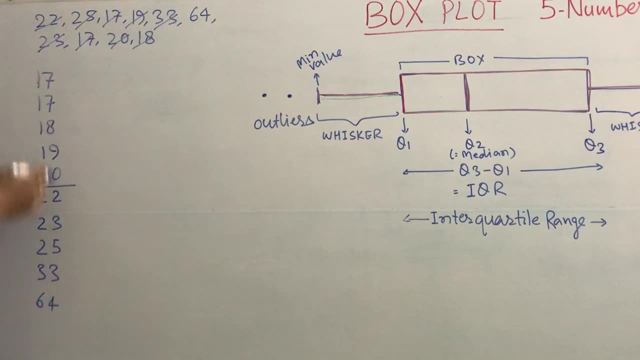 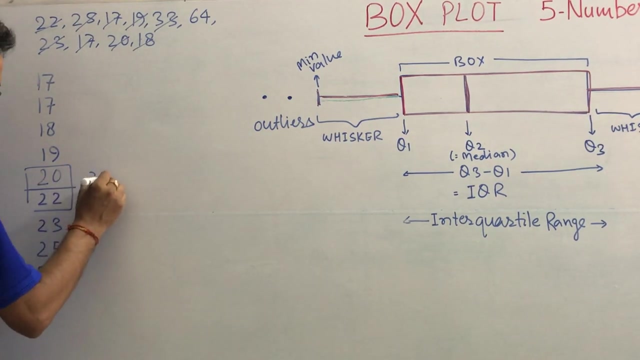 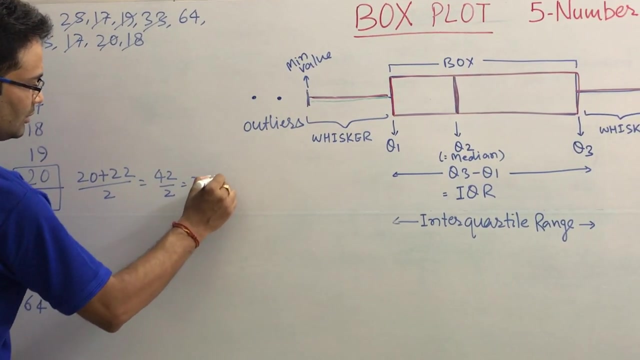 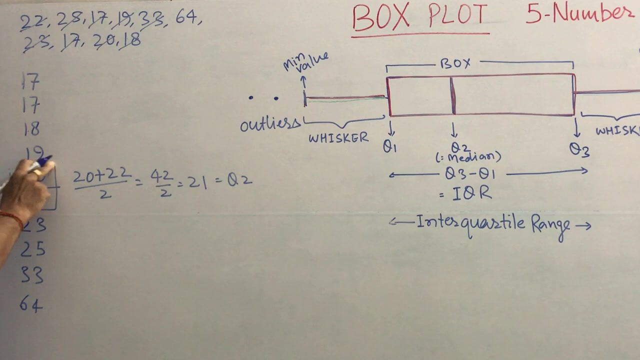 so median number will come. these two are the median number. so or other way, if this is the 10, you divide the 55, so this 2 is the middle number. so how you can get it: 20 plus 22 divided by 2, so to 42 by 2, 21. this is your quartile. how to get the quartile one. so here the half data in: 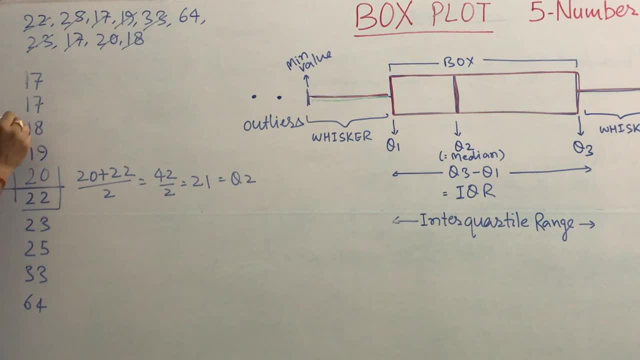 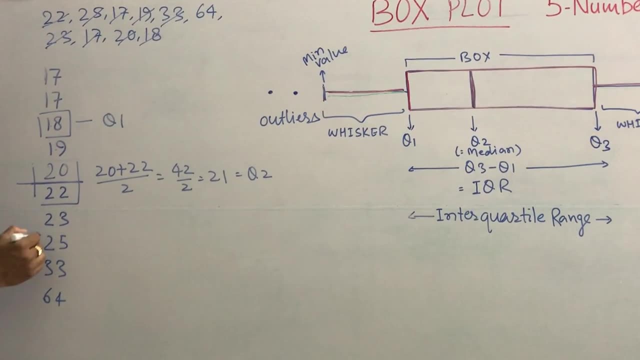 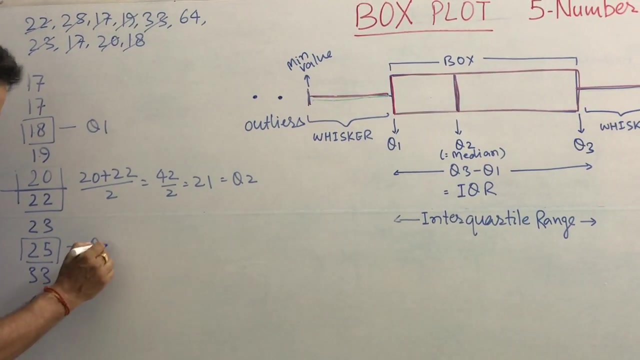 the half data. we have one, two, three, four, five, so we do one is the again QR and here half data. you still defeat 25p is the cube. so now we've got saw this is the que重o. we got the q1, q2, q3, but we 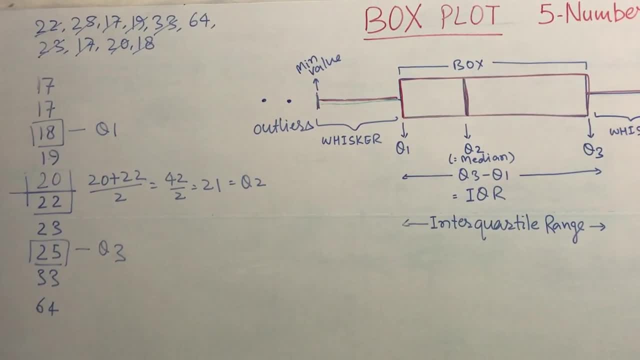 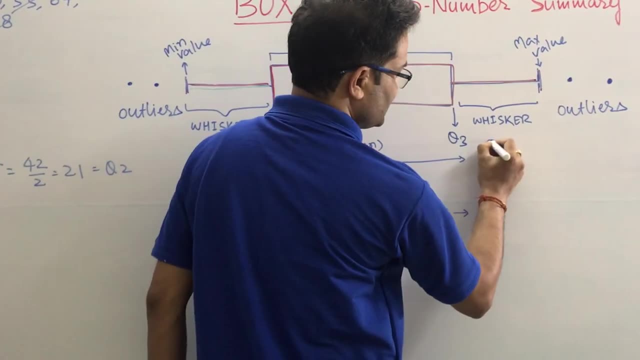 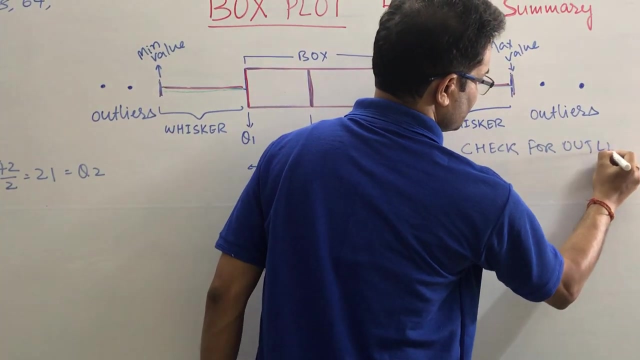 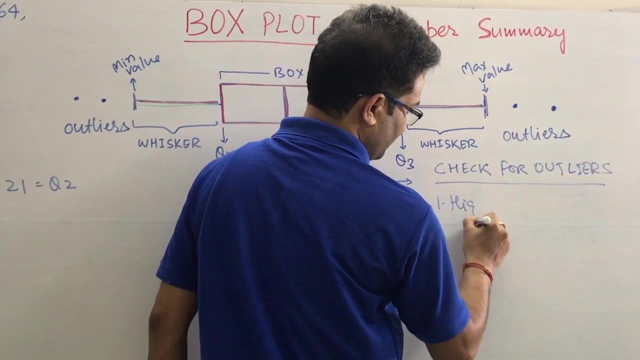 can't gerne that. this is the max mean all match. no, before that we have to check for the outlier, how I can save the options outlier, how i can save the options. so first check the four outliers. so we have two outliers, one is the higher outliers. if it is, 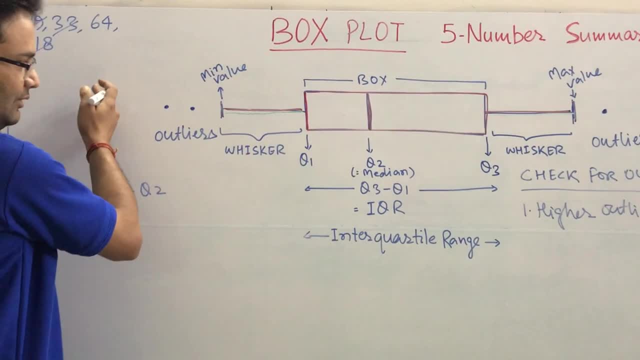 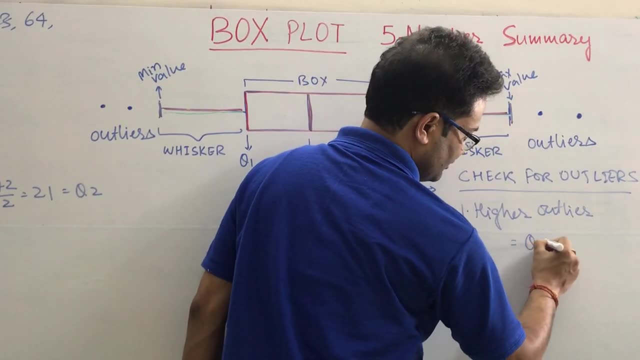 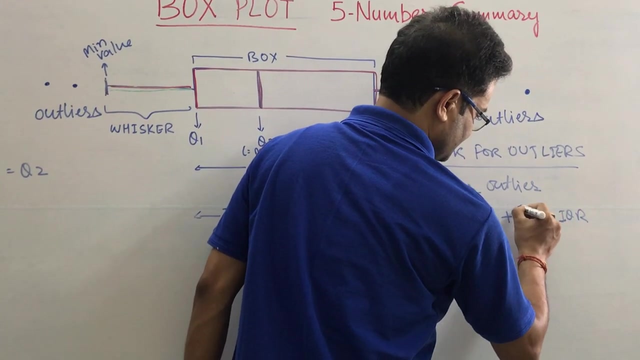 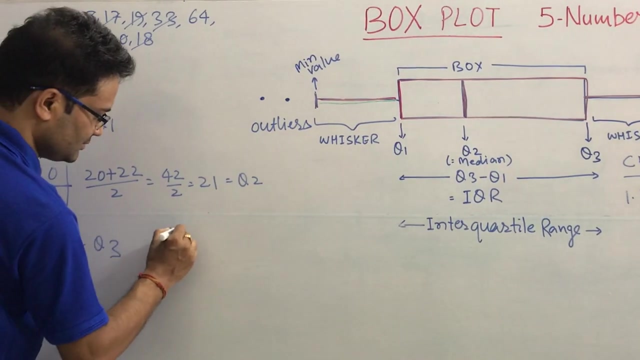 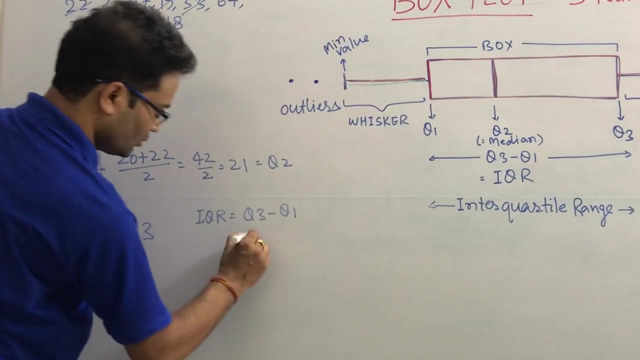 come out this side and we have the lower outlier, if it is come before the mean value. so how to get the higher outlier? formula is that q3 plus 1.5 into iqr. this iqr is this one. so in this case, what? how much iqr is this q3 minus q1? so what is q3? q3 is 25 minus q1 is the 18. so 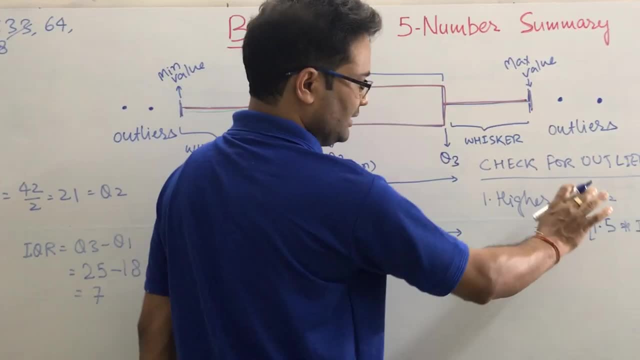 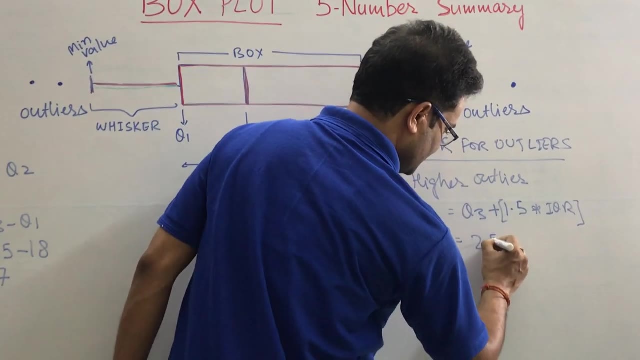 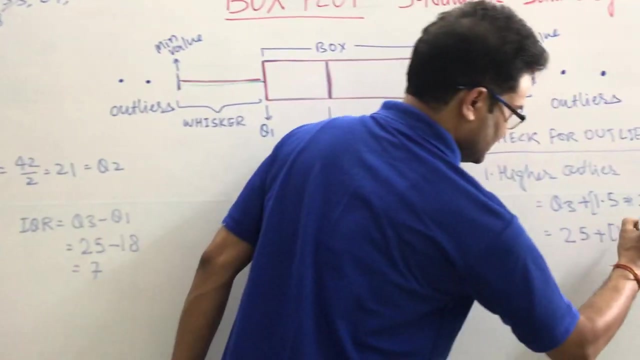 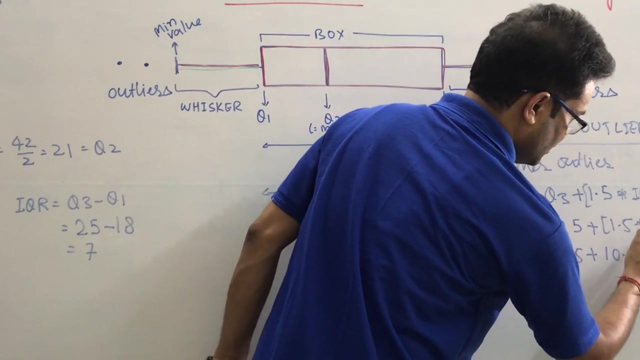 7 is the iqr. now we set here to find out the higher outlier. q3 is the 25, 1.5 in iqr is the 7. so put the 7 25 plus it will become the 10.5 quarter is equal to. 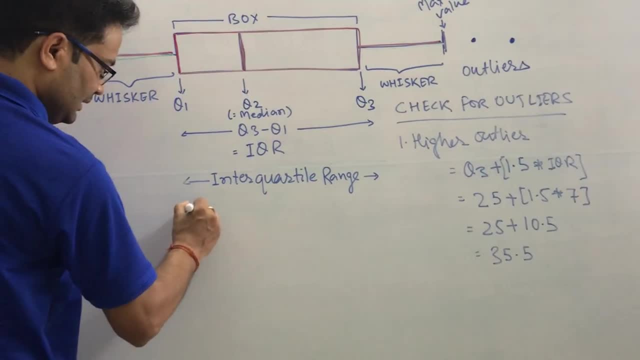 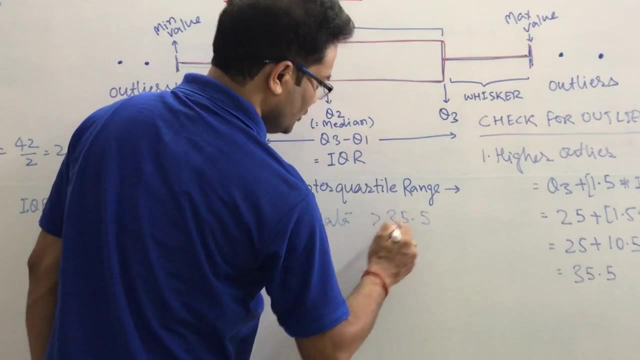 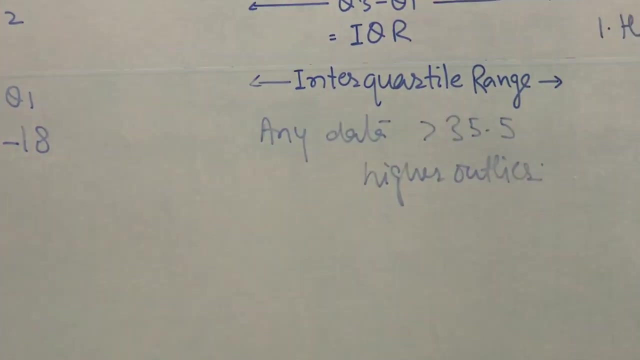 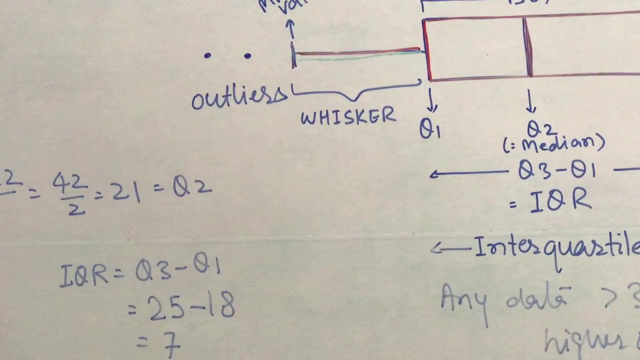 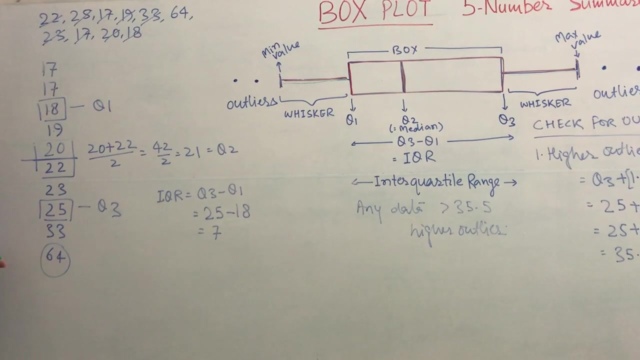 35.5. now, any data more than 35.5 would be the higher outlier. now check in your data set. any data is more than the 35.5. yes, 64 is the more than 35.5, so you can say this: 64 is the outlier. 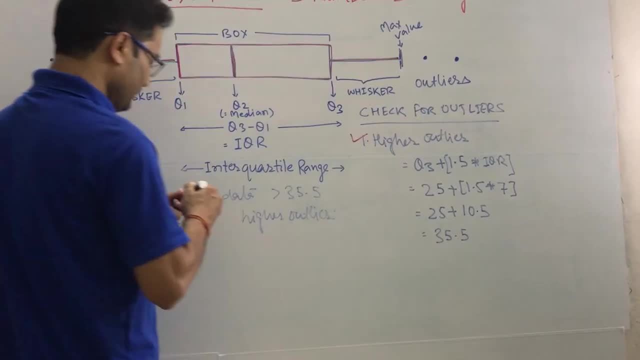 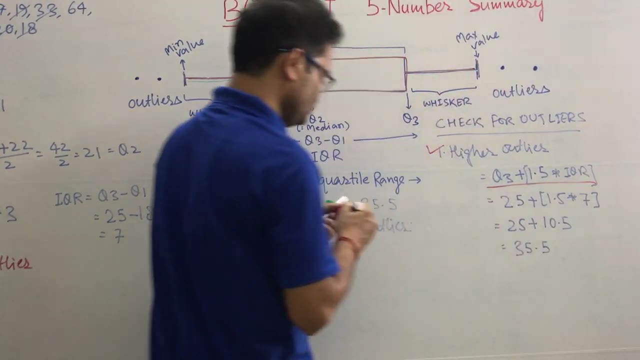 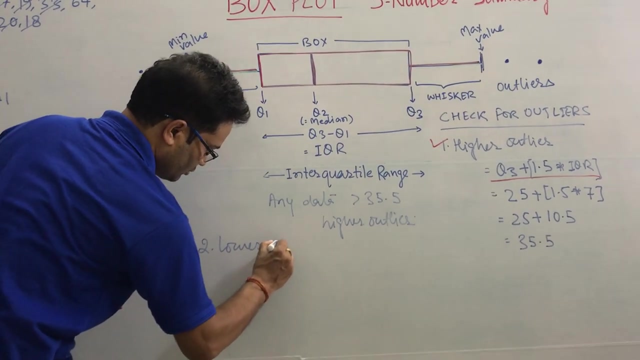 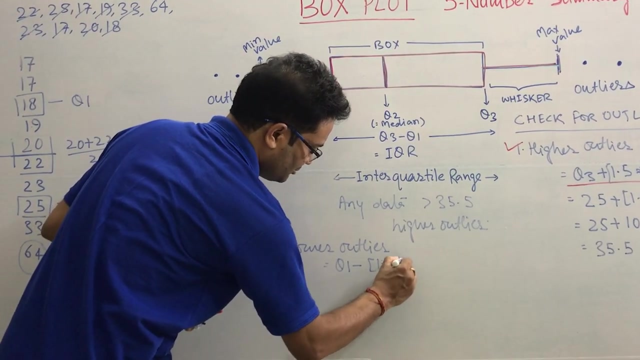 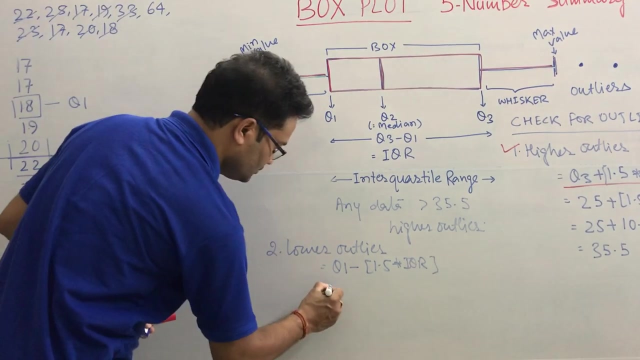 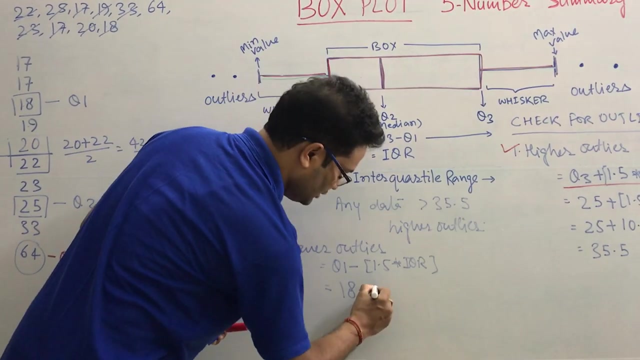 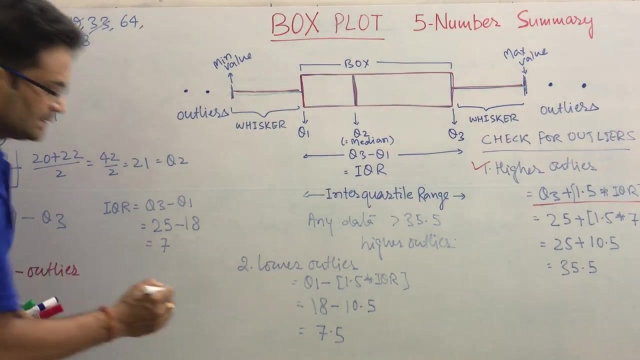 now, as we check the higher outlier, now we have to check the lower outlier. so formula was that the now check for the formula is q1 minus 1.5 into inter quartile range. so what is the q1? q1 is the 18. 18 minus 1.5 into iqr is equal to 10.5. so any value, any value less than 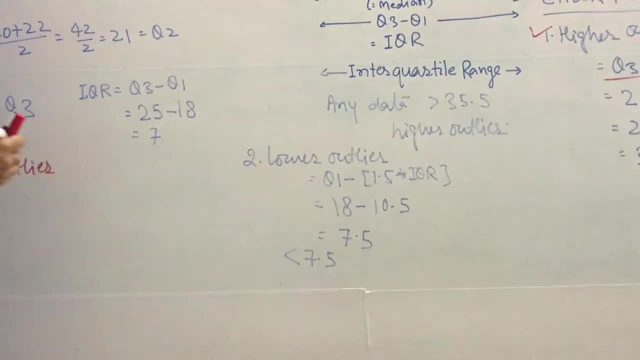 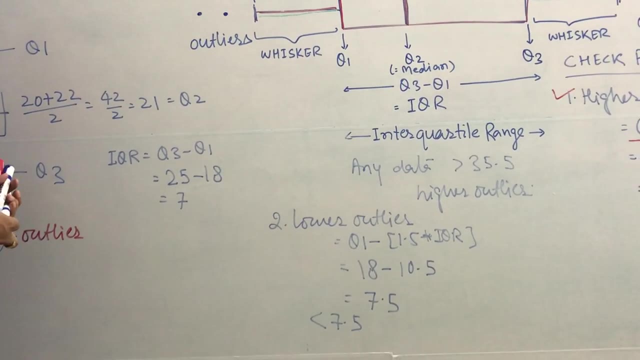 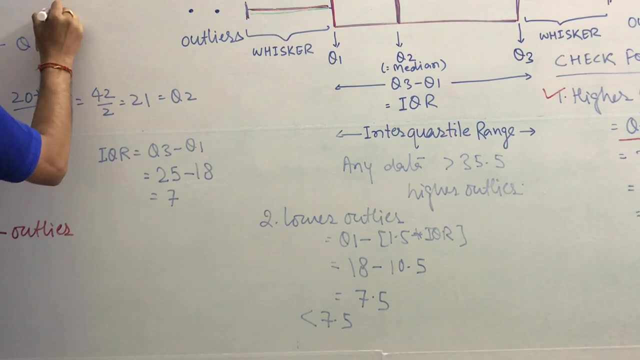 7.5 would be the lower outlier, but in this case we don't have any this data. so what we got from the complete picture, we got it: the q1 is 18, q2, 21, q3, 25, outlier 64. okay, so now 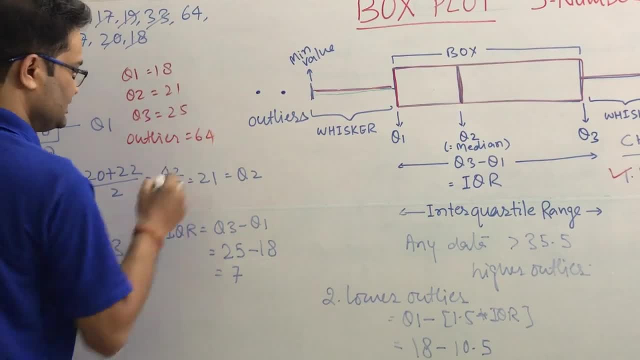 Ora, Let's see the outside. outlier 64. okay, so now. So what will we have in the complete picture? e1 is theKQ, 9 is the outlier S&A' Social law and all these things else, i تونят. and now look on the outside here, what is the q1? this one O word, and Q2, 21,, Q3,, 25- four, 64.. c-1, 85-65 pizzas, 24- silver, 65 keys. We do not have enough to have it. this people have the Q1 numbers itself. So now, 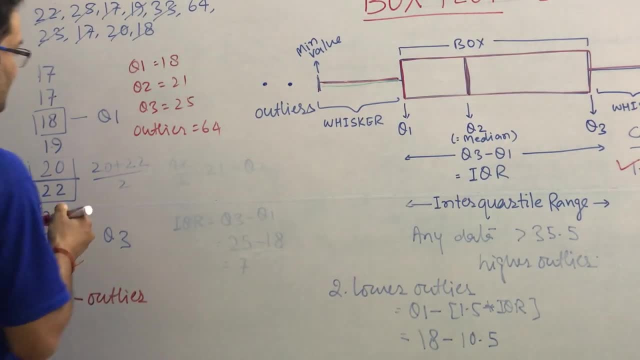 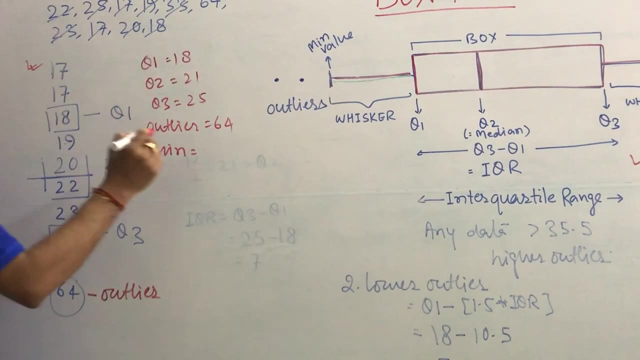 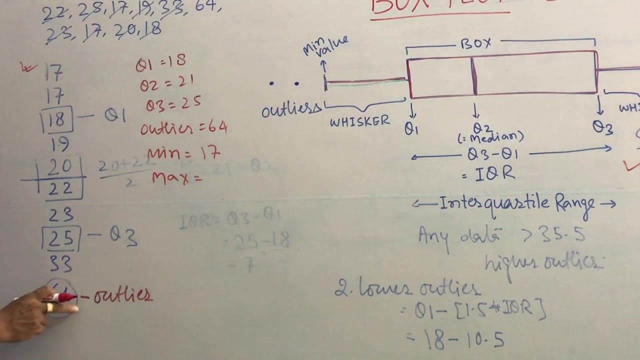 So what is the mean here? Mean is the lowest value and we don't have any outlier here. So this is the 17th. And what is the max value? Max is not the 64th, because 64 is the outlier, So 33 is the max.